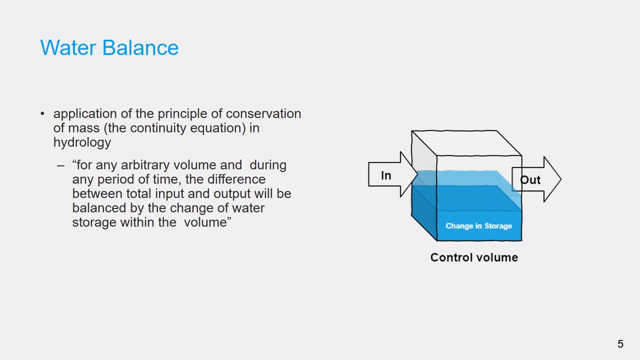 is used for operational management of reservoirs and for the compilation of hydrological forecasts for water management. Water balance studies provide an indirect evaluation of inexplicable water balance differences of different water sources with limited address, for example, in this particular case with the Drophugae. Interrest on monumental studying together was selfish. By doing so, their results could be summing up, often with increasing interest of the サ tn个 �رج précis, as well as the regression of choices of water resource in respect to cold moisture surfaces. Friday, Orester West. 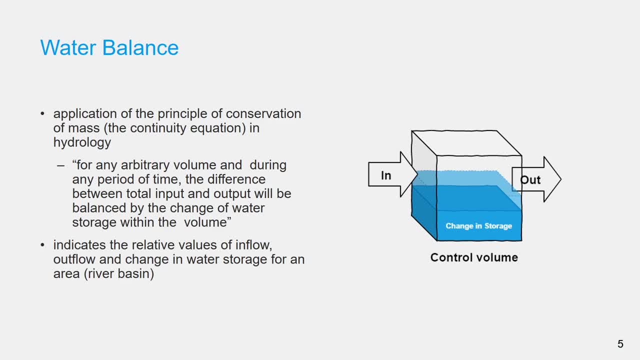 Following is how we use water balance strategies and problems that remind us to not smarter and less serious. In this phase, I would like to put, as a final EU, some slightly constructive questions for each particular group. an unknown water balance component? from the differences between the known components? 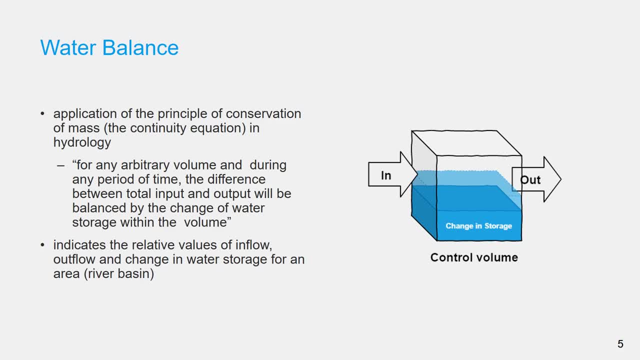 For example, long-term evapotranspiration from a river basin may be computed as the difference between precipitation and surface runoff. The study of water balance in hydrology is the application of the principle of conservation of mass, often referred to as the continuity equation. 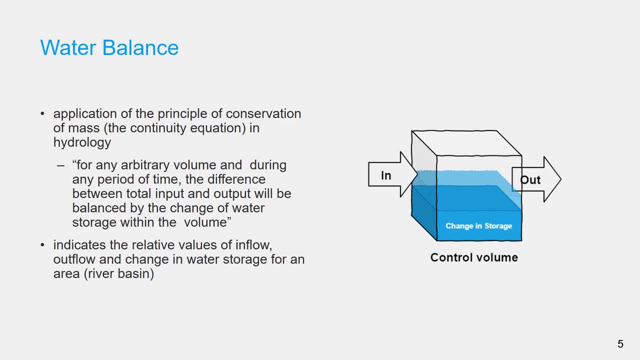 This states that for any arbitrary volume and during any period of time, the difference between the total input and output will be balanced by the change of storage within the volume. The water balance equation For any natural water area, such as the river basin or water body, indicates the relative importance or the relative 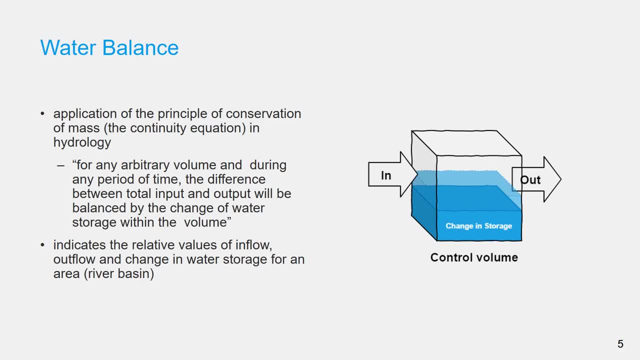 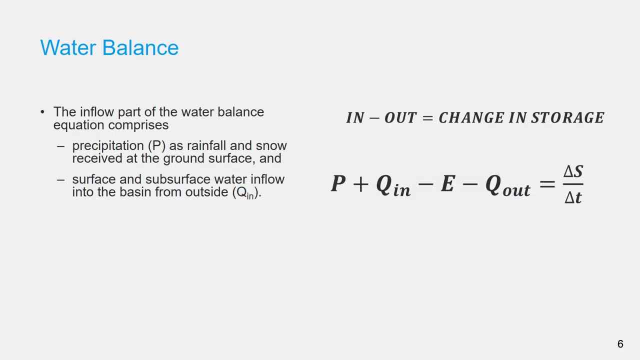 value of inflow, outflow and the changing water storage in the area In general. the inflow part of the water balance equation comprises precipitation as rainfall and the snow actually received at the ground surface and surface and subsurface water inflow. 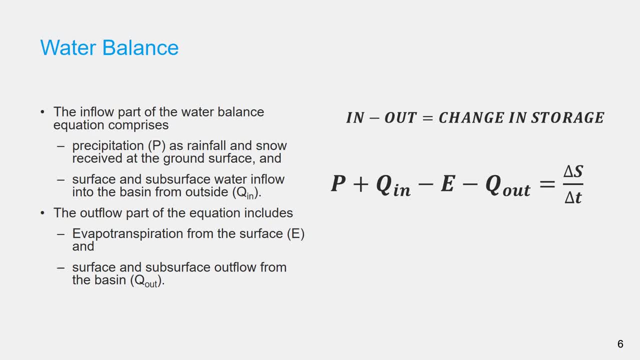 into the basin from outside. The outflow part of the equation includes evapotranspiration from the basin, surface and surface and subsurface outflow from the bed. When the inflow exceeds the outflow, the total water storage. An inflow less than the outflow results in decreased storage. 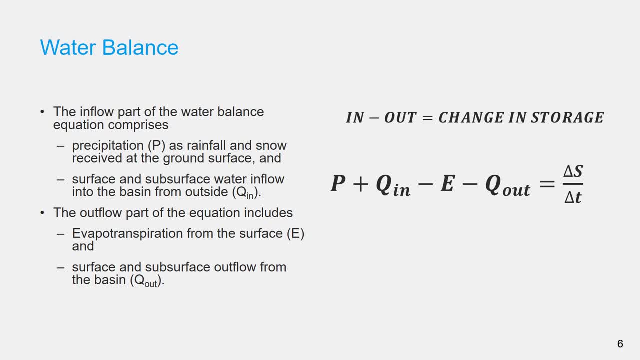 The water balance for any river basin or water body and any time interval in its general form may be represented by the equation shown in the slides. All the water balance components are subjected to errors of measurement. In any case, they don't ever reach a Adobe source path. while developing a general model, 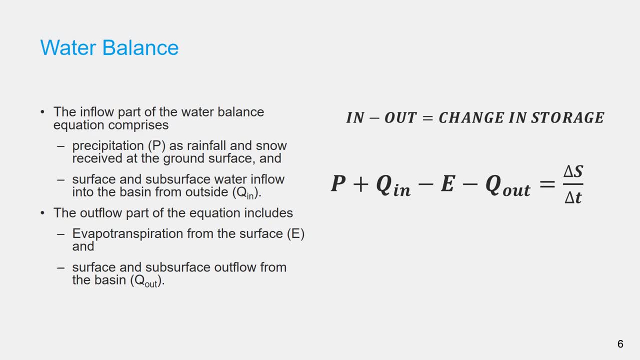 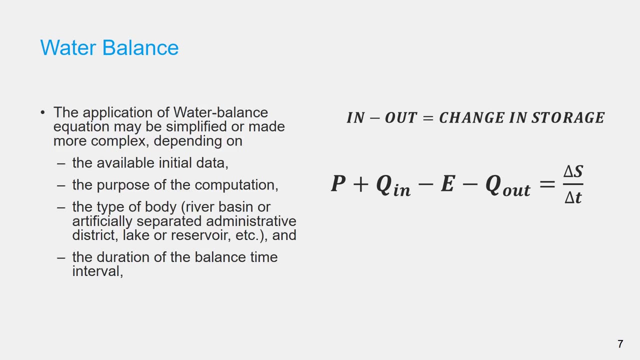 Form A demek lại removed a double way of soaking water in a single water tank or estimation and therefore they introduced uncertainty in the water balance estimation, which may produce differences in the left and right side of the equation. The application of the water balance equation may be simplified or made more complex, depending 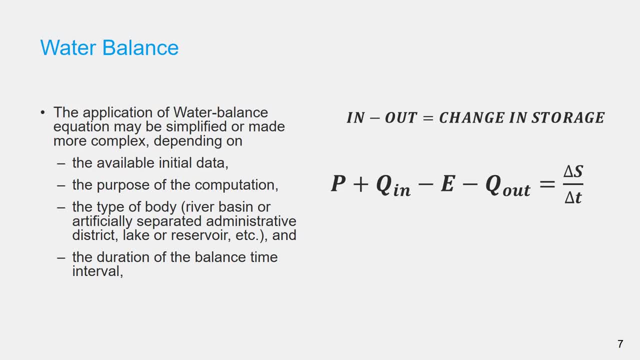 on several factors, including the available initial data. if we have data required to quantify all the input and output of the water balance equation. the purpose of the computation: for what purpose are we computing the water balance? the type of the body for which the 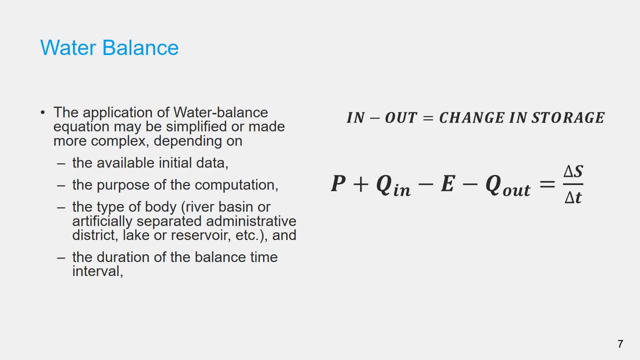 water balance is computed. is it a river basin Or artificial sea, And so on? Is it a parietal administrative region? Is it a lake or a reservoir? And the duration of the balance time interval. Are we computing the water balance for a yearly water balance, monthly, daily or different? 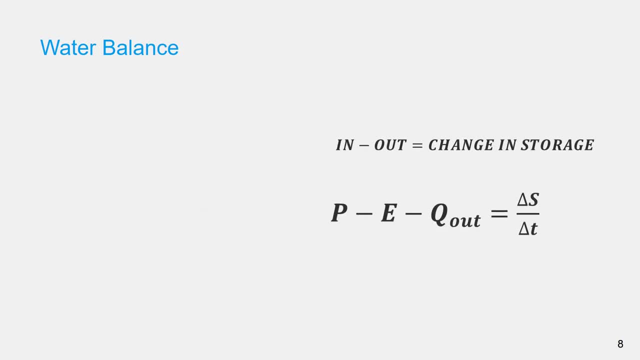 time step. In large river basins, subsurface water exchange with neighboring basin is assumed to be zero. No surface water inflow into a river basin with distinct catchment divide, Of course assuming no artificial diversions from other basins. In this case, the water balance equation is simplified as precipitation as the only inflow. 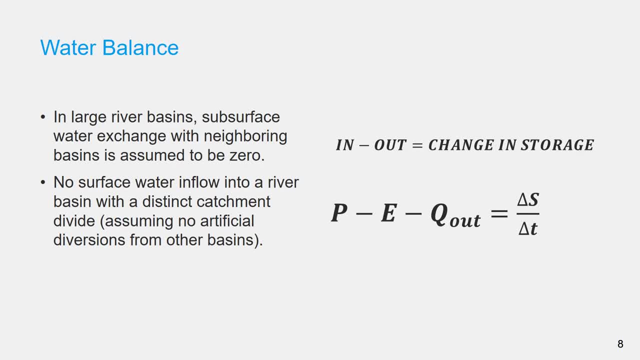 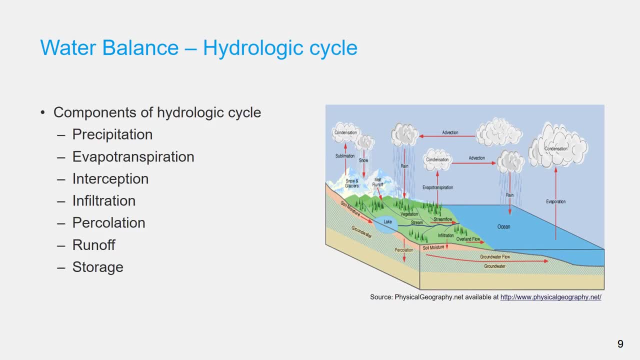 and evapotranspiration and discharge out of the basin as outflow components. Thank you for your attention. Water balance method can be used to evaluate the components of the hydrologic cycle. The hydrologic cycle is a conceptual model that describes the storage and the movement. 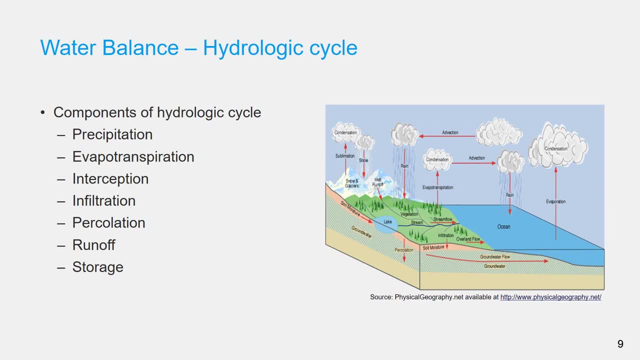 of water between different spheres of the earth, which are biosphere, atmosphere, lithosphere and the hydrosphere. The biosphere includes water. The hydrosphere includes water. The hydrosphere includes water. The hydrosphere includes all life on earth: plants, animals and humans. 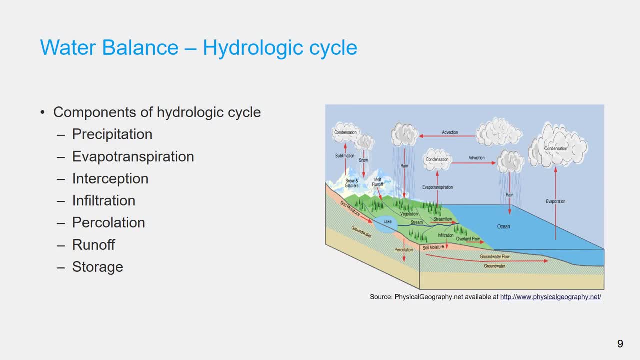 The hydrosphere includes all water on the planet, the oceans, the lakes, rivers, groundwater, rain clouds, glaciers and ice caps. And the atmosphere includes all the air above the surface of the earth all the way to space. 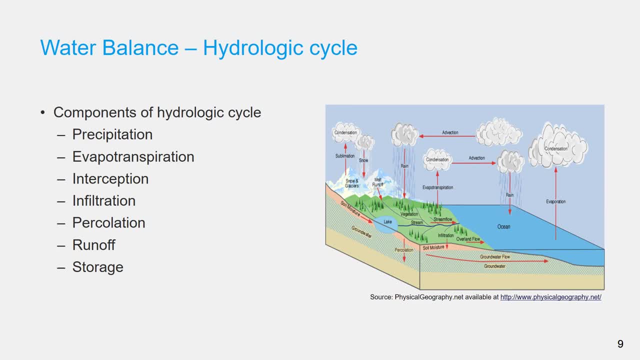 And the lithosphere includes the Earth's crust and the upper part of the mantle. Water can be stored in any of the following reservoirs In the atmospheres: oceans, lakes, rivers, soils, snow fields and groundwater. And water moves from one reservoir to another via three major pathways. 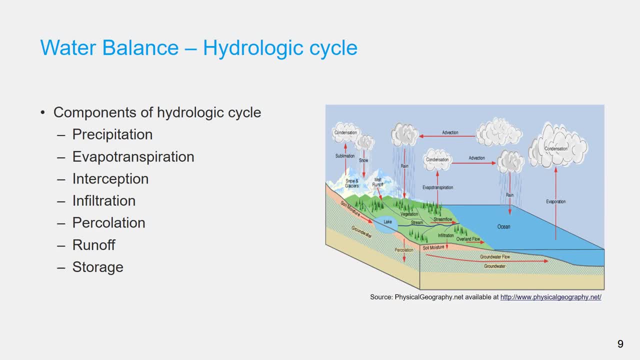 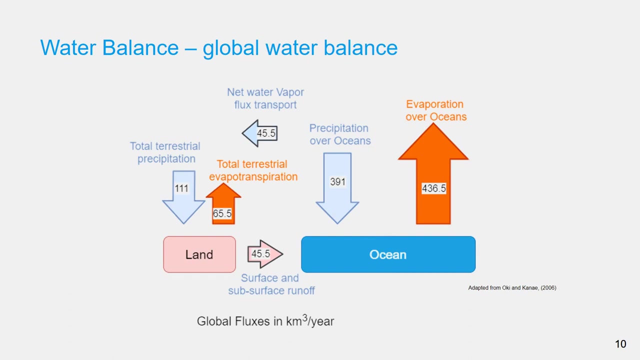 These are precipitation on the ground, on the Earth's surface and on the ocean, evapotranspiration and vapor transport- movement of vapor from one place to another. Oakey and Kane estimated the global water balance in their paper titled Global Hydrological. 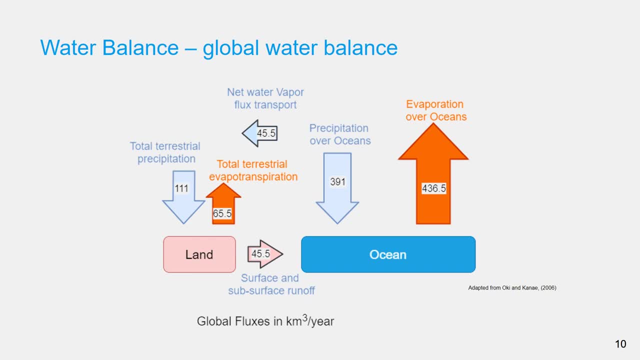 Cycles and Wallet Water Resources in 2006.. Looking at their estimates, we can observe that there is more precipitation on the land surface than evapotranspiration and more evapotranspiration than precipitation on the ocean. The differences between precipitation and evapotranspiration are balanced as surface. 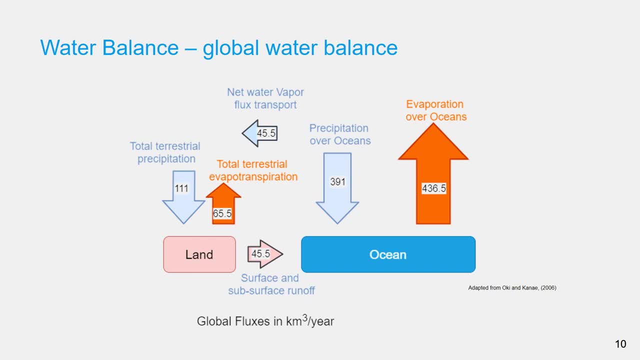 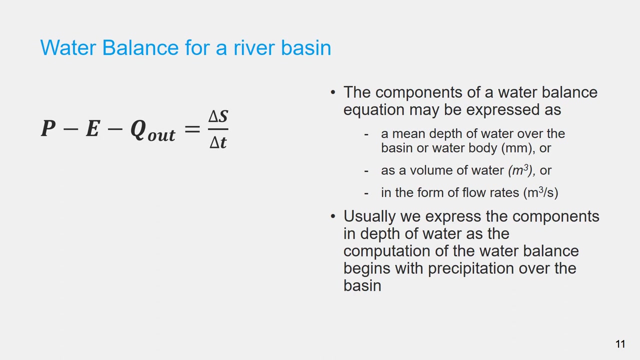 and subsurface, runoff from the landmass to the oceans And, as net water vapour flows from the oceans to the land surface, We have seen that the components of water balance for rivers are different. river basin are precipitation, evapotranspiration, runoff from the basin and change of water. 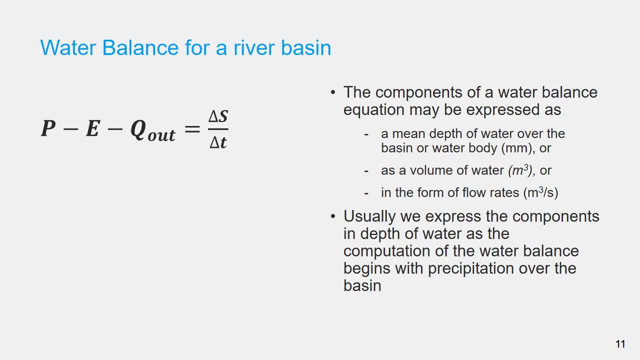 storage within the basin. These components may be expressed in three different units. They can be as mean depths of water over the basin area in mm of water depth, or as total volume of water in m3, or as flow rates in m3 per second. 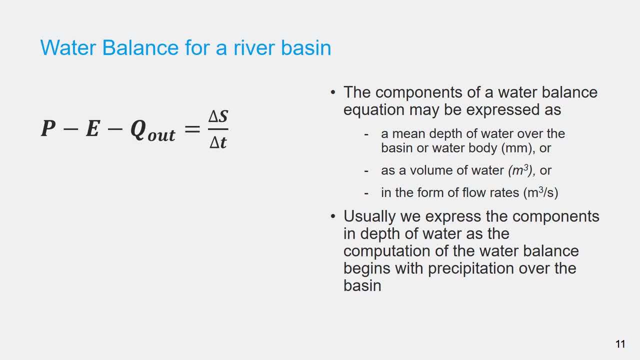 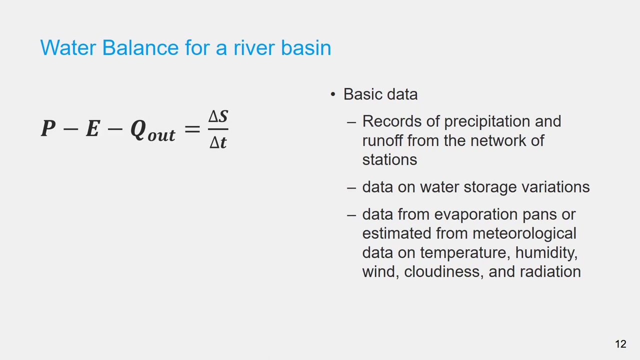 Expressing the water balance components in flow rates is convenient for many water management communications. However, as the computation of water balance usually starts with the computation of mean precipitation over a basin, the other components are different. They are usually also expressed as depths of water. 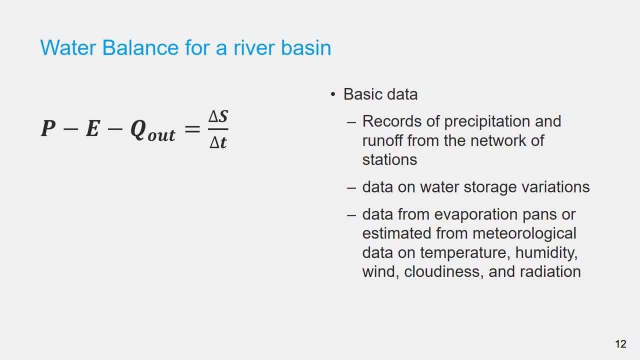 Records of precipitation and runoff from network of stations are the basic data for computation of the water balance components of a river basin for long-term periods. To compute the water balance for individual years, seasons or months, it is necessary in addition to have data on water storage variations in the basins. 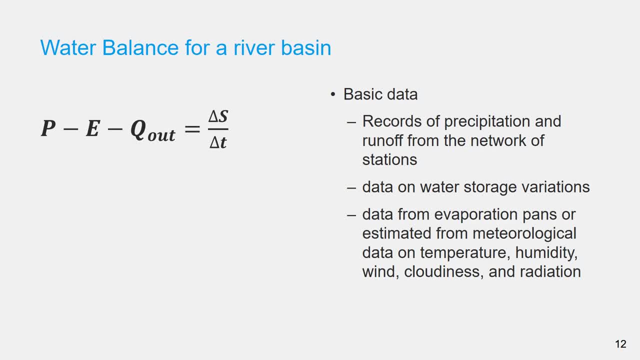 These are obtained from snow surveys, observations of soil moisture, water level fluctuations in lakes and groundwater fluctuations in wells. To compute evapotranspiration, it is desirable to have data from evaporation pans or tanks with meteorological data on temperature, humidity, wind, cloudiness and radish, which 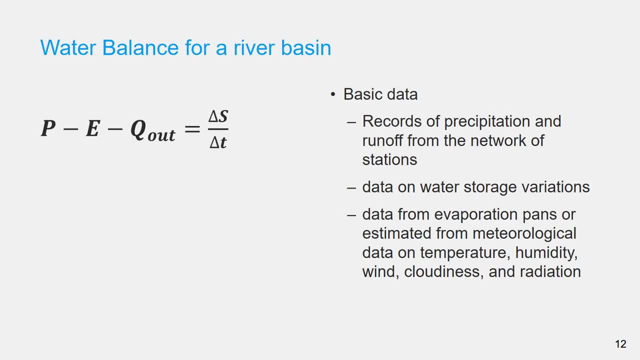 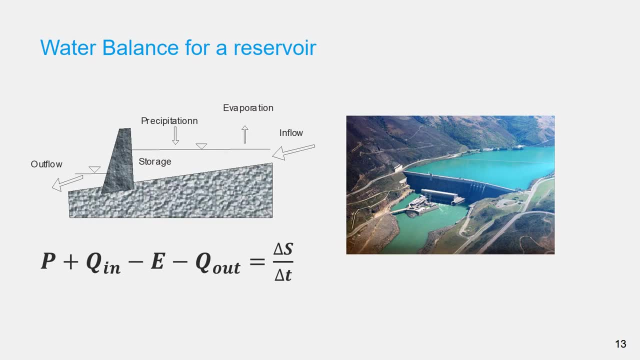 are used to compute evapotranspiration. The water balance equation for reservoirs and lakes for any time interval may be written as the equation shown here, where p is the precipitation on the surface of the lake or reservoir and e is the evapotranspiration from the surface of the lake. 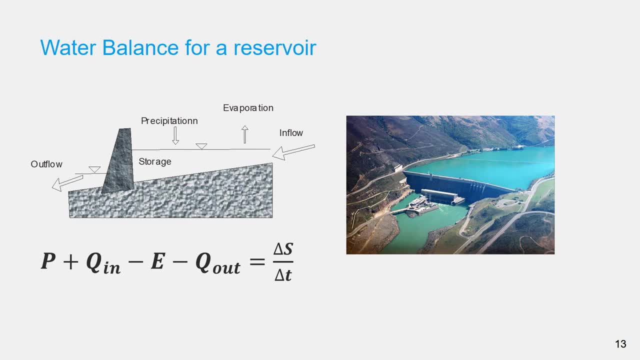 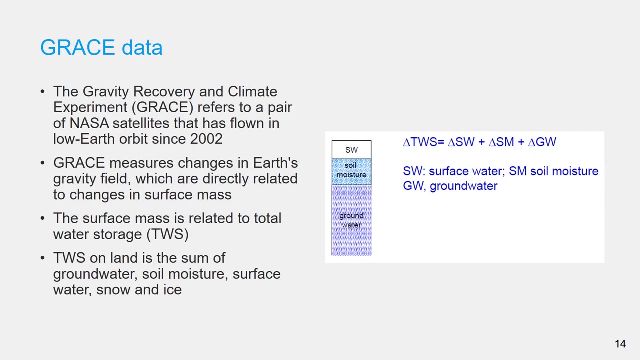 The inflow to the reservoir includes any surface and subsurface inflow and the outflow includes outflow from the reservoir, including groundwater outflow and percolation through the dam. For most of the main components of a water balance equation are available, we can compute. 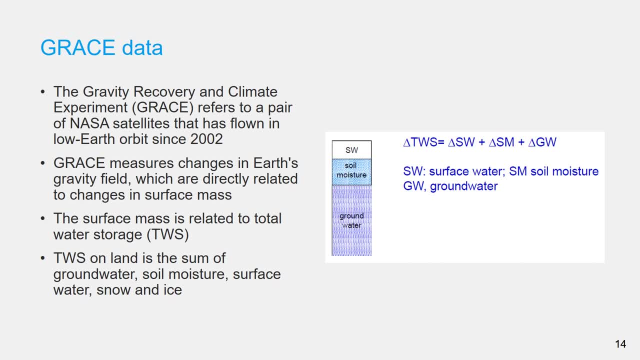 the water balance of a river basin using remote sensing data. The remote sensing data we need for water balance computation are maps of precipitation, evapotranspiration and change of storage. Precipitation and evapotranspiration data can be obtained from various remote sensing. 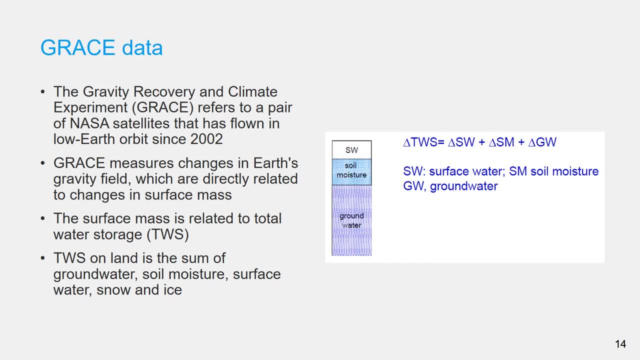 products. In addition to these products, we need estimates of change of water storage. To estimate change of water storage in a river basin, we use GRACE data. The Gravity Recovery and Climate Experiment refers to a pair of NASA satellites that have flown in low-Earth orbits since the year 2002 to measure changes in Earth's. 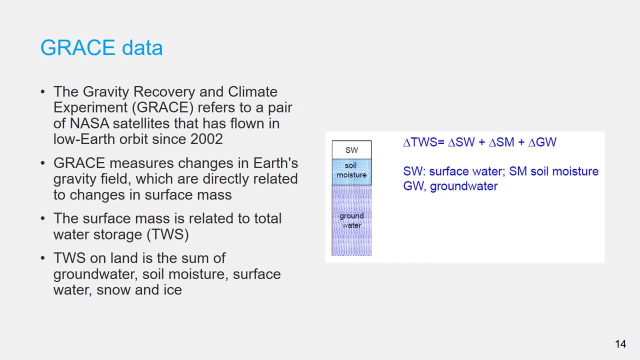 gravity field, which are directly related to changes in the surface mass, And the surface mass signal largely reflects total water storage. Total water storage on land surface is the sum of all the groundwater, soil, moisture, surface water, snow and ice. 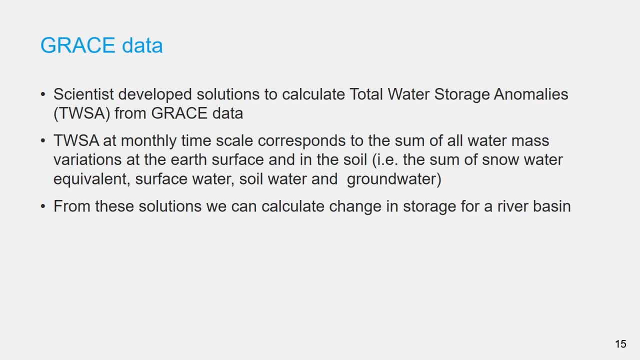 Scientists develop solutions. Scientists develop solutions To calculate total water storage anomalies from GRACE data. GRACE solutions provided as total water storage anomalies at monthly time scale correspond to the sum of all water mass variations at the Earth's surface and in the soil. 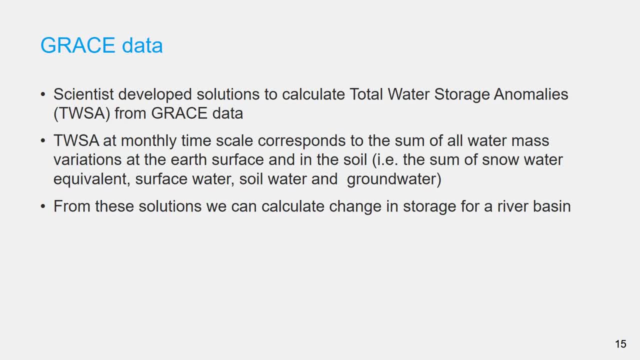 That means it includes the sum of snow water, equivalent surface water, soil water and groundwater. That means it includes the sum of snow water, equivalent surface water, soil water and groundwater. From these solutions we can calculate changing the storage for a river basin. 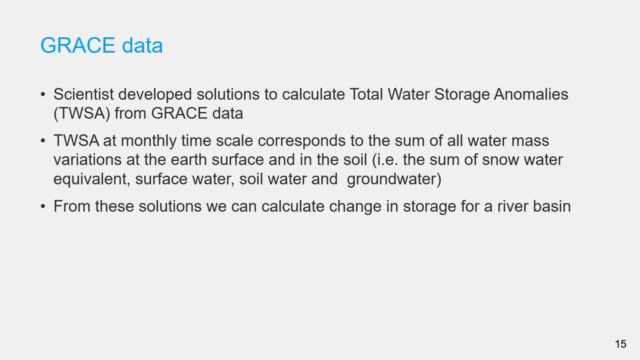 We can also¡¡¡¡¡¡¡¡¡¡¡¡¡¡¡¡¡¡¡¡¡¡¡¡¡¡¡¡¡¡¡¡¡¡¡¡¡¡¡¡¡¡¡¡¡¡¡¡¡¡¡¡¡¡¡¡¡¡¡¡¡¡¡¡ éner. 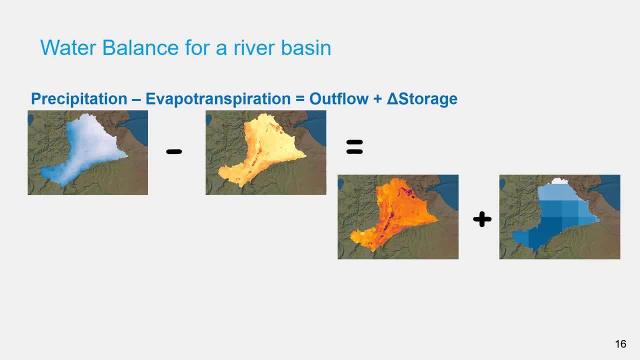 over the Однако¡¡¡¡¡¡¡¡¡¡¡¡¡¡¡¡¡¡¡¡¡¡¡¡¡¡¡¡¡¡¡¡¡¡¡¡¡¡-__ side of the belt". 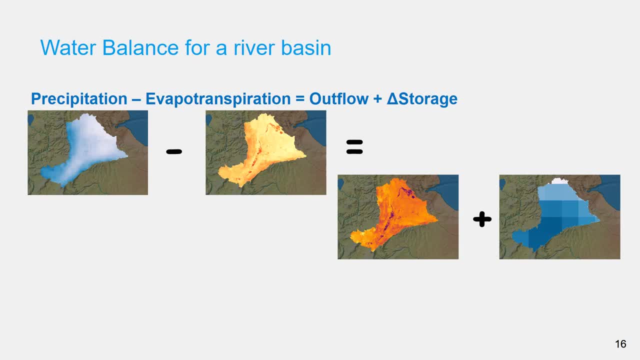 Thank you for sticking with us to this discussion. Thank you¡¡¡¡¡¡¡¡¡¡¡¡¡¡¡¡- All right, I hope I could help someone- nobody else. We can evaluate if the water balance can be closed or not using data from remote sensing. 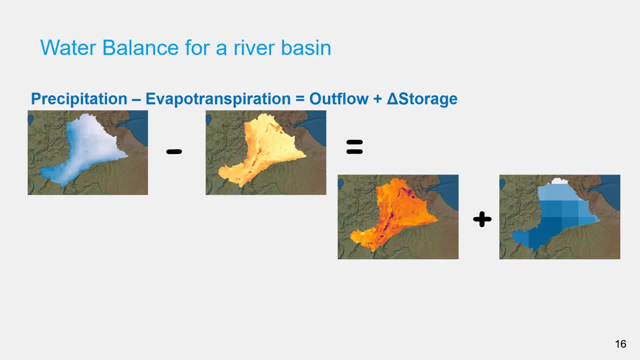 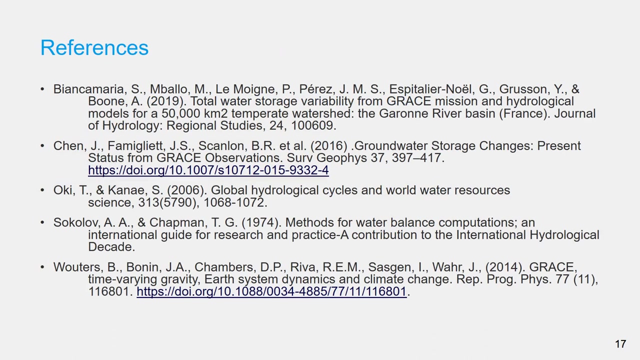 products In the water balance computation exercise. we use remote sensing products to compute water balance for Awashi River basin in Ethiopia, using VAPOR data for precipitation and evapotranspiration and GRACE data for changing water storage. Some of the reference materials I used to prepare these slides and for you to read more. 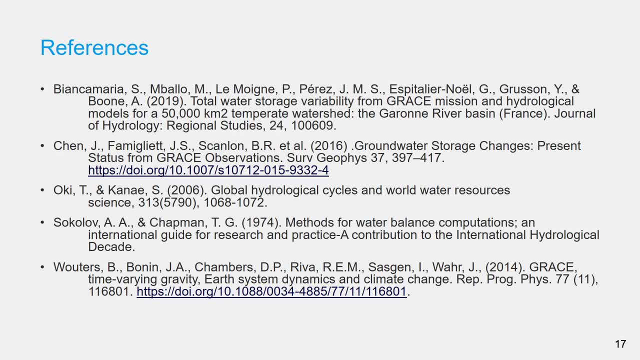 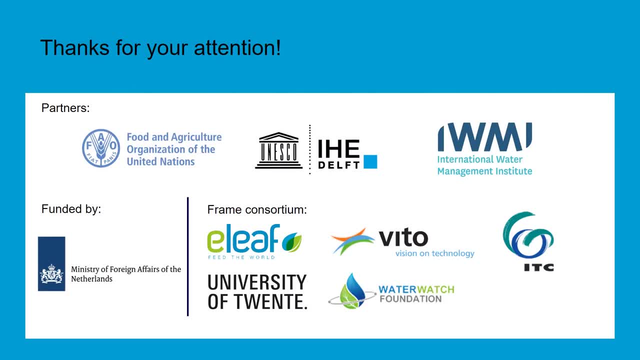 about. the topics covered are listed in this slide. Thank you for your attention and I hope you gained some insight about water balance and how we can compute water balance from components of hydrologic cycle. Hope to see you in the next unit. Till then, goodbye.